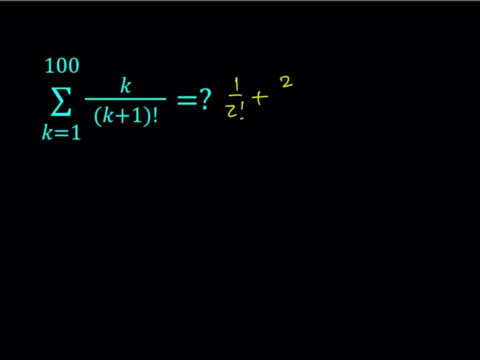 factorial- Great. And then if I replace k with 2, I get 2 over 3 factorial, And then I get 3 over 4 factorial. This is going to go on all the way up to 100. divided by 101 factorial, Obviously 101. 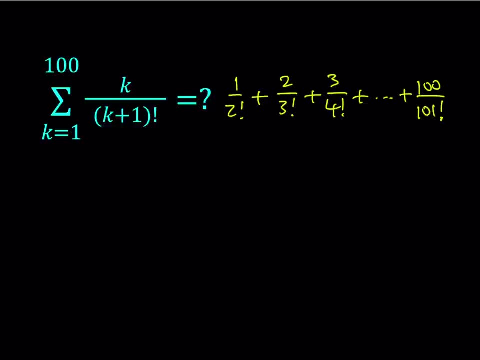 factorial is a very, very large number. It's huge, And I don't think you want to evaluate this And I don't think you want to make a common denominator, which would be obviously 101 factorial- Maybe smaller, but you kind of have to think about the least common multiple of all these. 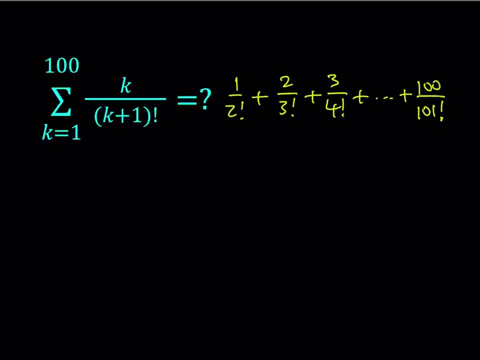 numbers. Anyways, that's going to be huge. So we're going to be using a different approach Now. when we're solving problems for integer solutions or when we're manipulating rational expressions, a common strategy that we use is to manipulate. 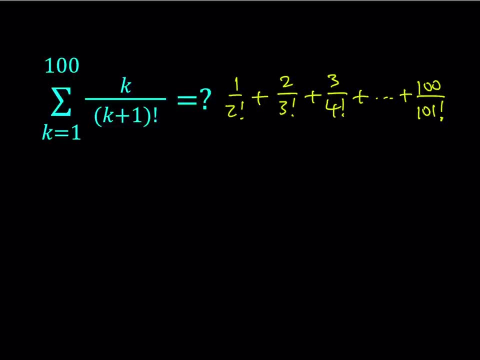 the numerator so that we can separate this into pieces and make it a telescoping sum. What is a telescoping sum? A lot of terms are going to cancel out, leaving us with a few terms here and there. Let's go ahead and do that, And the trick involves manipulating the k, Since I have k plus 1. 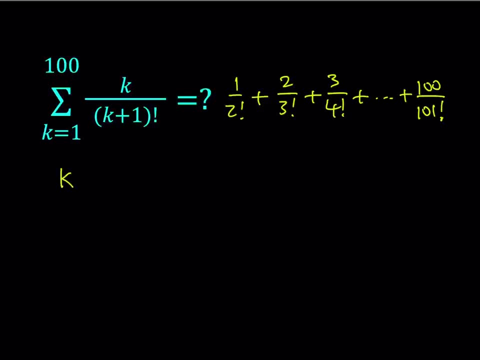 factorial. at the bottom I would like to add 1 and subtract 1.. So write the k as k plus 1 minus 1, legitimate right, And then, of course, divided by k plus 1 factorial. Now we're going to split. 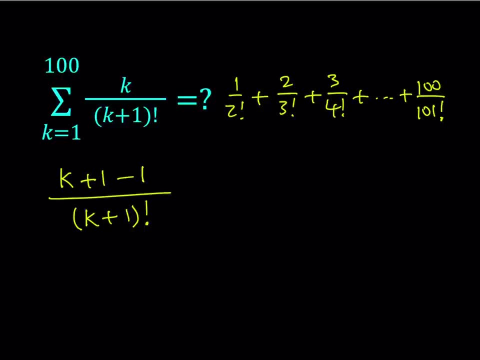 it up into two fractions and hopefully make it a telescoping sum. So in that regard I can write it as k plus 1 divided by k plus 1 factorial minus 1 divided by k plus 1 factorial. So far you may not have seen the trick or what we're going to do next yet, but here's what it is. 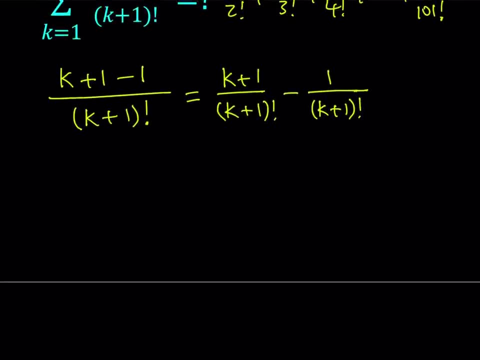 I have a k plus 1 and k plus 1 factorial. What is that supposed to mean? Well, k plus 1 divides k plus 1 factorial. In other words, they have a common factor because I can write k plus 1 factorial. 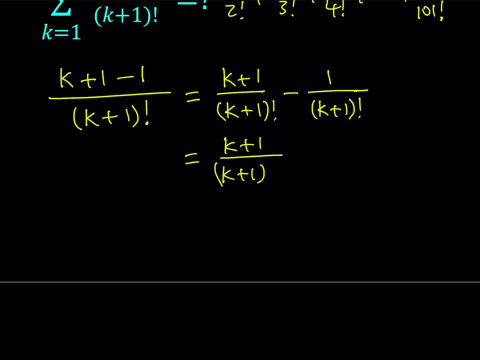 as k plus 1 times k factorial, And isn't that awesome? That's what's really awesome about factorials: that you can really factor them and simplify them. So we can go ahead and simplify k plus 1.. That leaves us with k plus 1.. So we can go ahead and simplify k plus 1.. That leaves us with 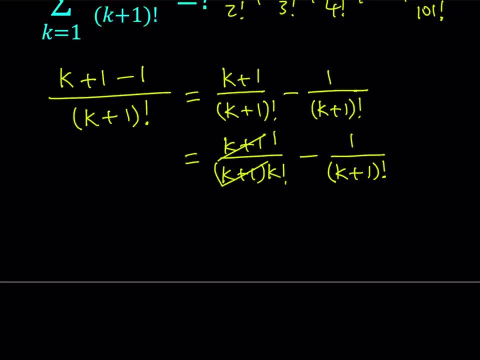 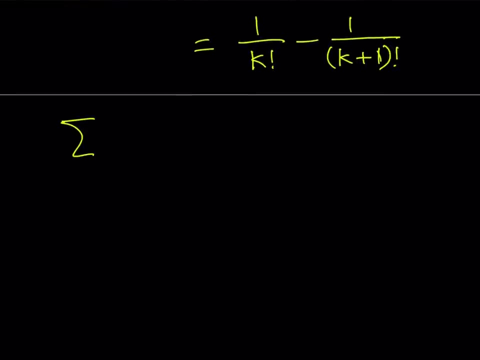 1 over k- factorial minus 1 over k plus 1: factorial. I'm going to go ahead and rewrite this. Here's a cleaner version. This is what I have And, as you know, this is a telescoping sum, So I would like to evaluate this. k equals 1 through 100. And you know that the sigma allows. 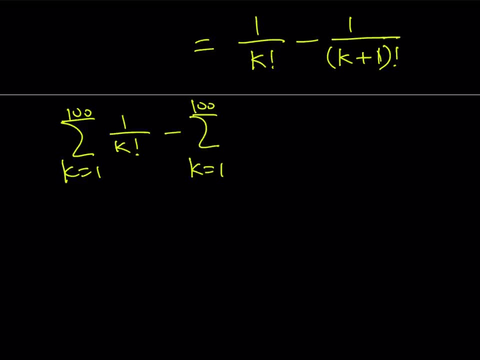 us to separate these two things, right? So if you have a sum which is also a difference in this sum, then you can separate them, And this makes it a little easier So you don't really have to deal with like what cancels out what so on and so forth. I'm going to deal with two sums. The first 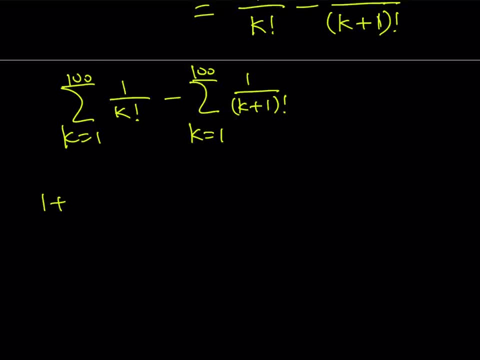 sum is 1 over 1 factorial, which is 1.. And then I'll get 1 over 2 factorial, 1 over 3 factorial, so on and so forth, all the way up to- uh-oh, don't do that, Desmos. Okay, I mean notability. 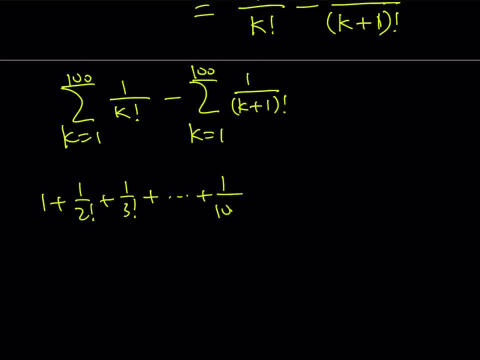 plus dot, dot, dot all the way up to 1 over 100 factorial. This is my first sum, So I'm going to subtract the first sum And from this I'm going to subtract the second sum, which is 1 over 2. 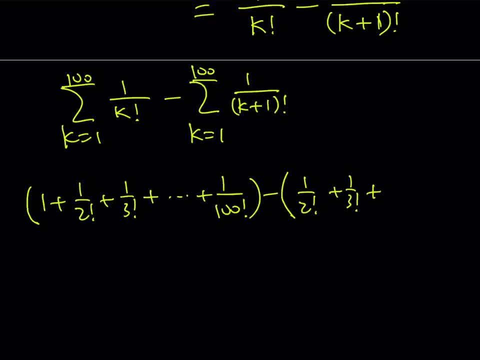 factorial plus 1 over 3 factorial plus, so on and so forth, all the way up to 1 over 100 factorial. And then we have the last term as 1 over 101 factorial. I wrote two terms so that you can see. 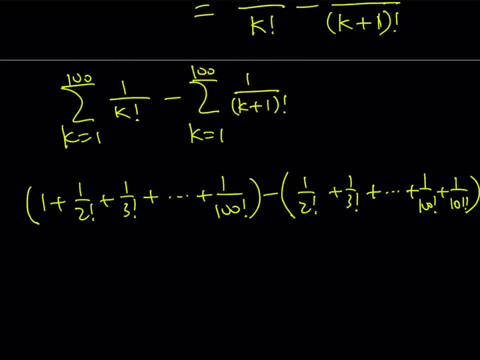 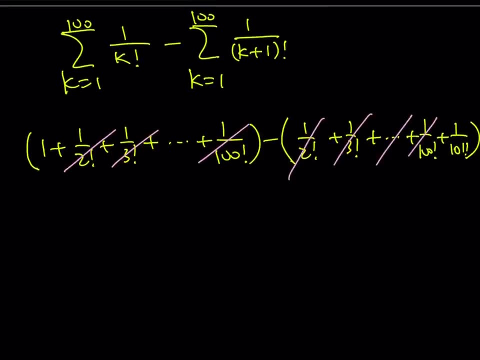 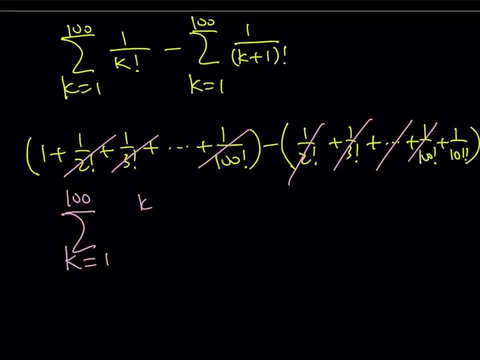 what cancels out easily. Now, here, between 2, I mean 2 through 2,, 2 through 100, everything is going to cancel out. And now we're going to end up with two simple terms. So our expression, which is: k equals 1 through 100, k over k plus 1 quantity. 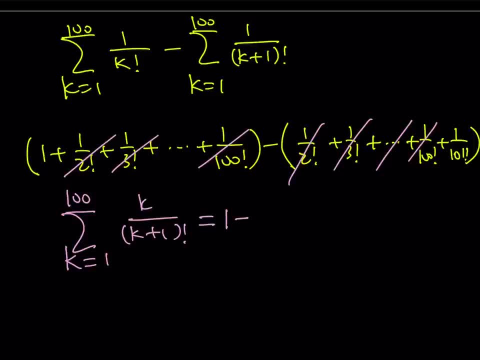 factorial can be written as 1 minus 1 over 101 factorial. Obviously, you can make a common denominator and write it as 101 factorial minus 1 divided by 101 factorial, And basically you can write it like this, And this is going to be very close to 1,. 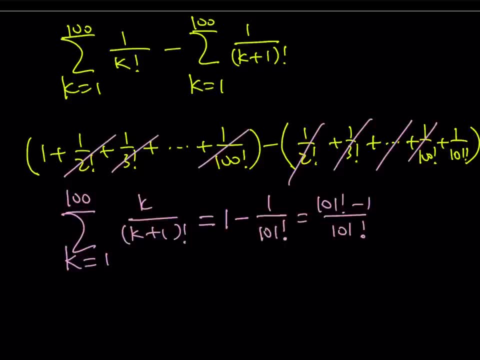 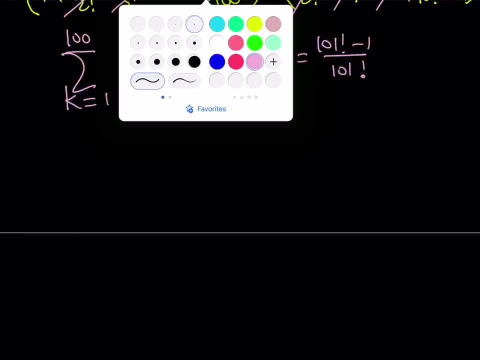 because 1 over 101 factorial is a very small number. So if you subtract it from 1, you're going to be very close to 1.. And this brings us to the end of this video. Well, thank you for watching. I hope you enjoyed it. Please let me know. Don't forget to comment, like and subscribe.